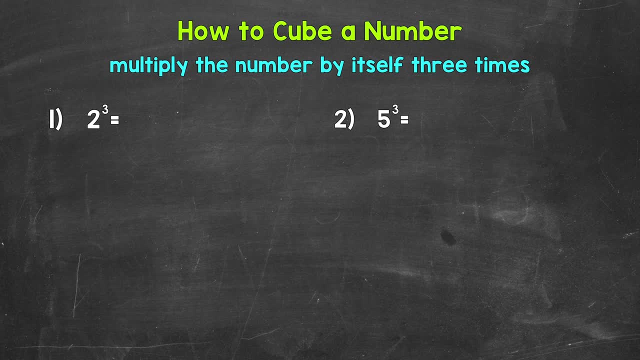 Let's jump into our examples and see exactly what this looks like, Starting with number one, where we have two cubed. Now, when working with exponents, the bigger number to the left is called the base. For example, in number one, this two is the base. 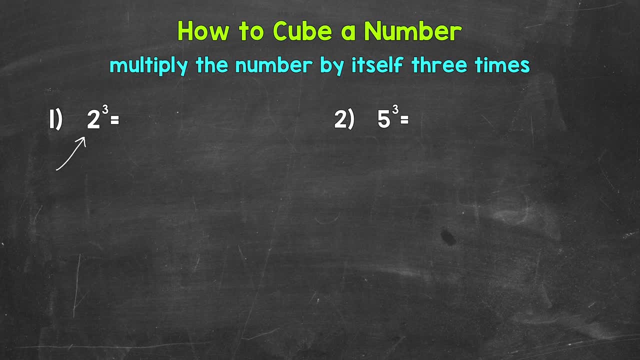 The smaller number to the right is called the exponent. This three is the exponent in number one. So whenever we see an exponent of three we are cubing a number and we can say that number is a number. For example, in number one we can say two cubed. 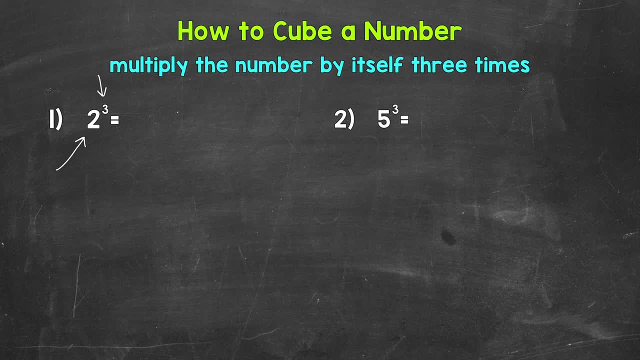 Now this means that we multiply the number by itself three times. We multiply that base by itself three times. Let me rewrite two cubed down below. So two cubed equals two times two times two. We take that base of two and expand it out three times. 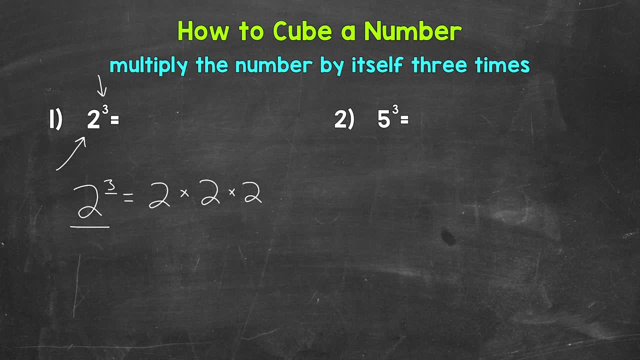 Two times two, Two is four times two is eight. So two cubed equals eight. Before we move on to number two, I do want to mention why we call it cubing a number. If we take a look at a cube, we can see why we call it cubing a number. 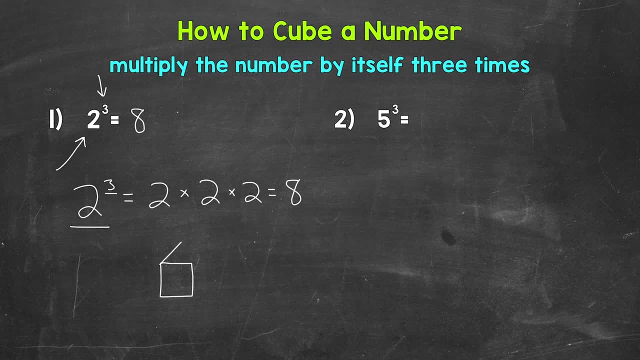 For example, if we were to take a look at a cube that was two by two and we wanted to find the volume of that cube, we would want to do length times width times height, which would be two times two times two, which is just two cubed. 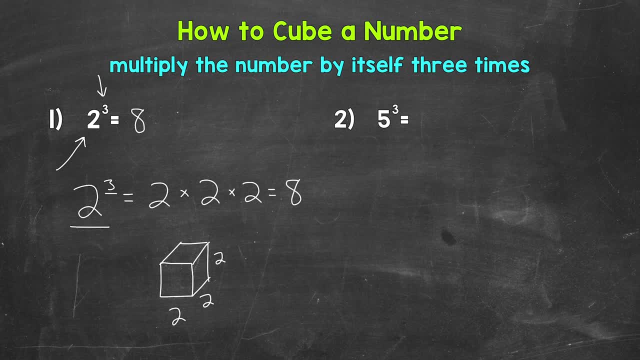 We can cube an edge length to find the volume of a cube. So you can see the relationship between cubing a number and the volume of a cube. Let's move on to number two, where we have five cubed, which means five times five times five.